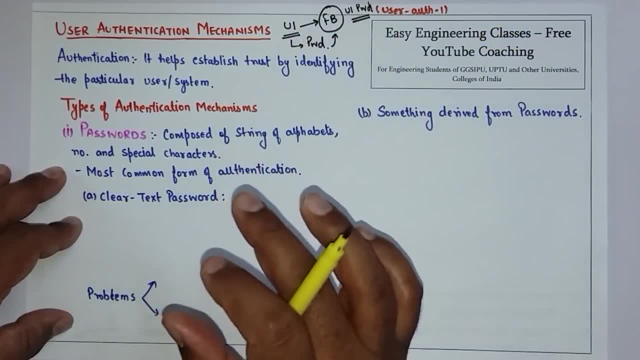 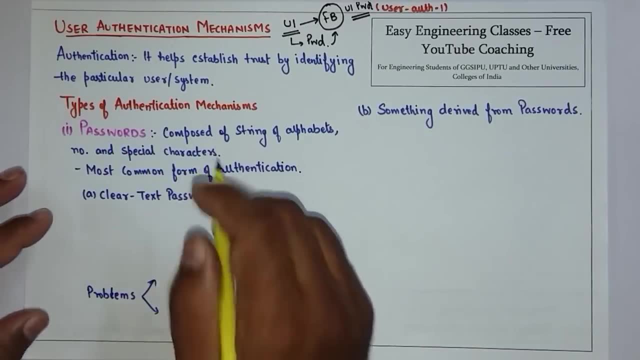 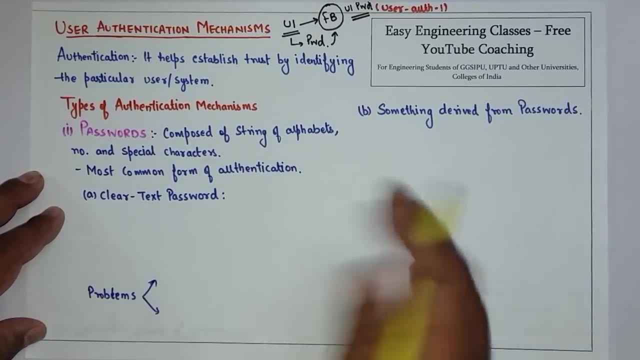 If both are the same, that means this is the authentic user. So authentication is the process that helps establish trust by identifying the particular user or system. Now there are different types of authentication mechanisms. First of all, in today's video lecture, we will learn about passwords. 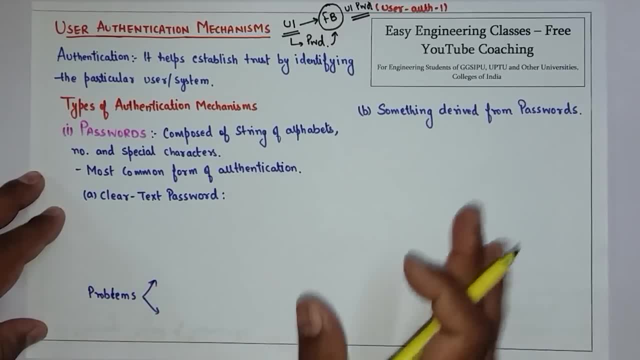 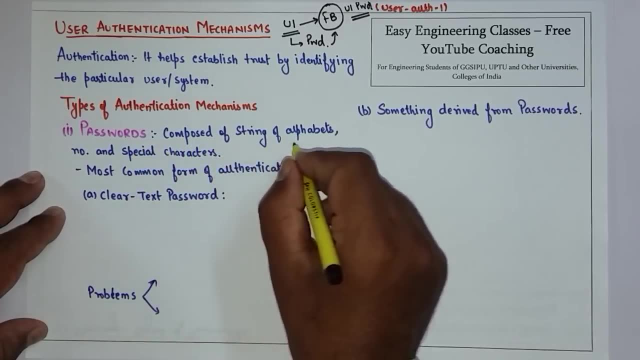 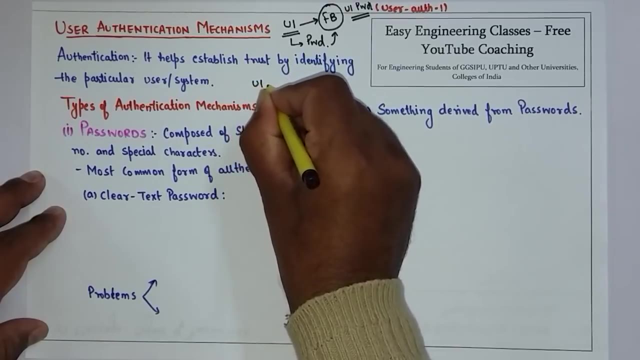 Passwords are the simplest kind of authentication mechanism that you can use. It is very simple: The password composed of string of alphabets, number and special characters, Like if you are a user u1.. What password can a user u1 set? 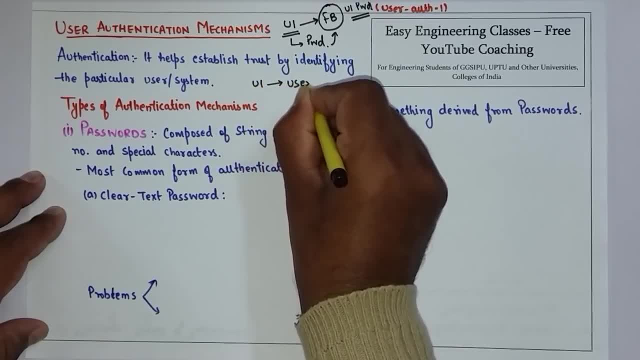 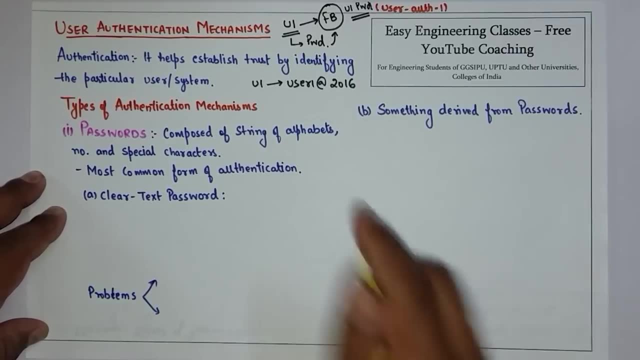 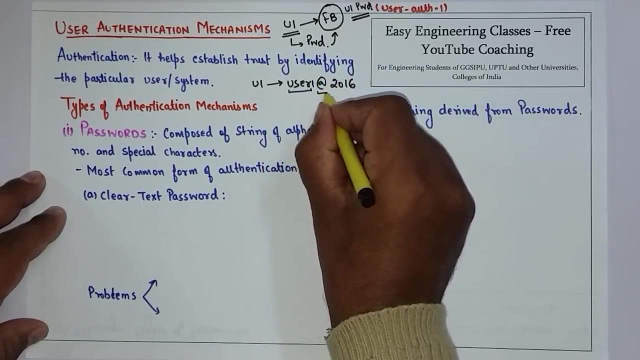 Suppose, user 1 at the rate 2016.. So what is there in this password? There are string of alphabets, special characters and numbers. So this is the password for user 1.. And password is the most common form of authentication, which is used every day. does not matter if 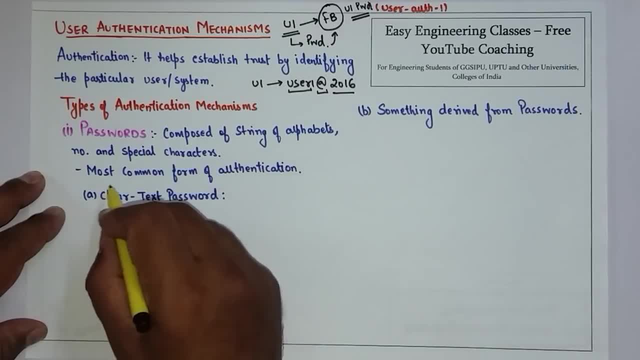 you are using Facebook or Instagram, So I will be using nucleos. I have used a nucleos, So I will be using nucleos. I have used a nucleos. I have used a nucleos. I have used a nucleos. 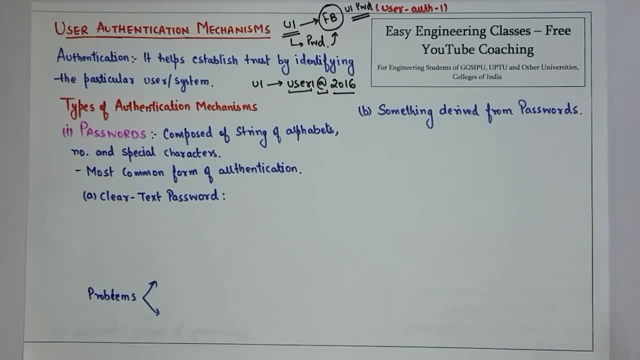 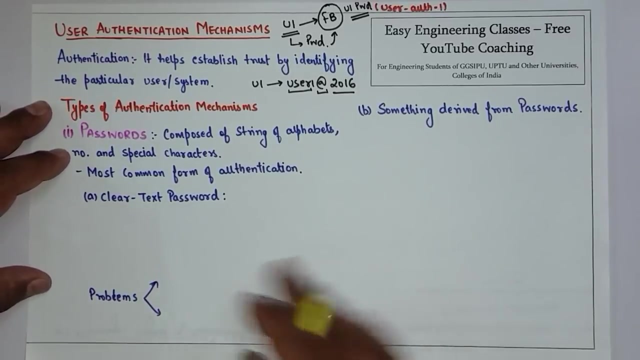 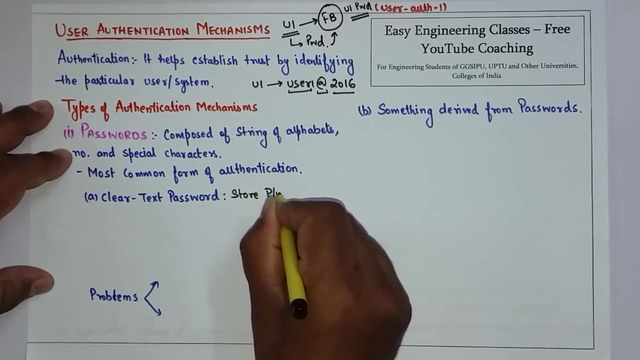 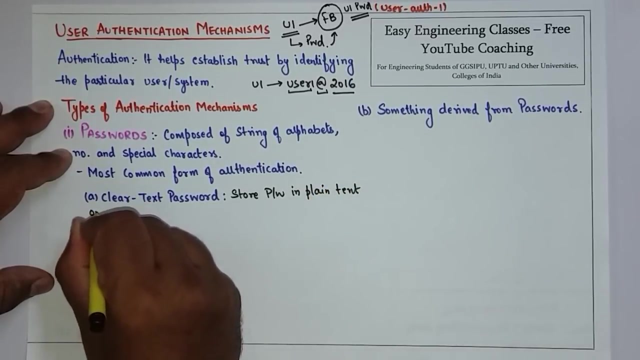 in the world. now we will see different kinds of password mechanisms that are used and the problem with the clear text passwords and how to solve that problem. sobhse pehle jo password ka mechanism hai, that is clear text password. clear text password ka. kya matlab hai in this? we store the password in plain text on the server. 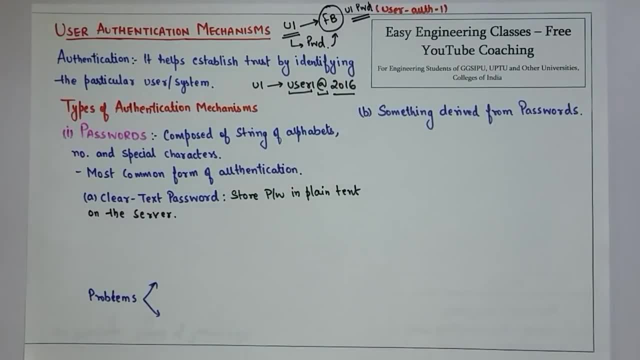 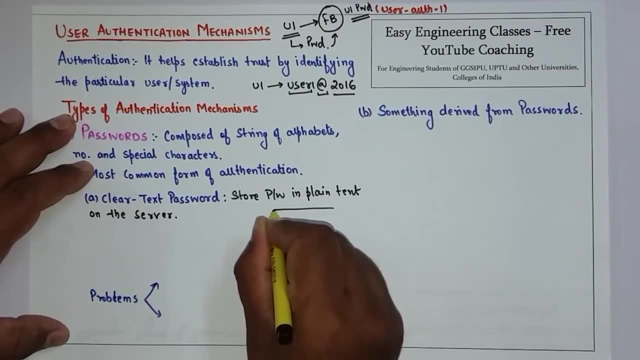 hum server ke upper apne password ko simple plain text ki form mein store karte hain. jaise agar hum yap ek pura system bana, ke meh apko dekhaata hu, iska simple plain text ki form mein store karte hain. 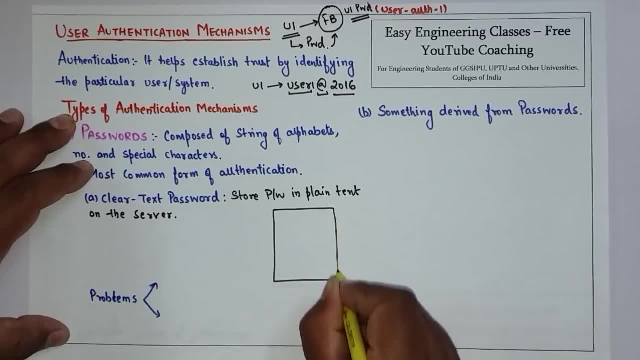 Suppose this is the server. we have a server. What will happen to this server? your details, User ID and corresponding passwords? Suppose U1's password was user1 and user5's password was user5. So this is the server containing user IDs and passwords. Now, here we have a client. 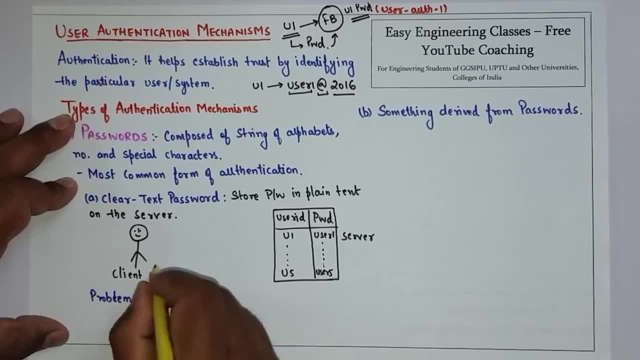 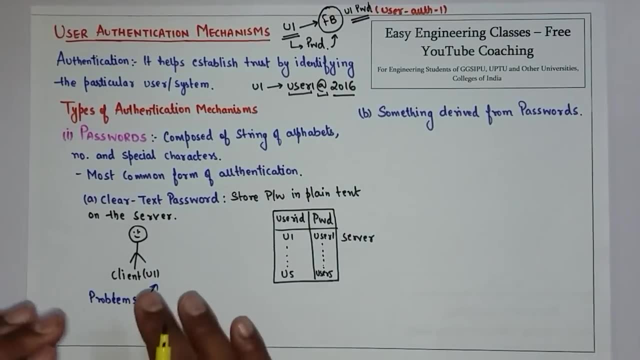 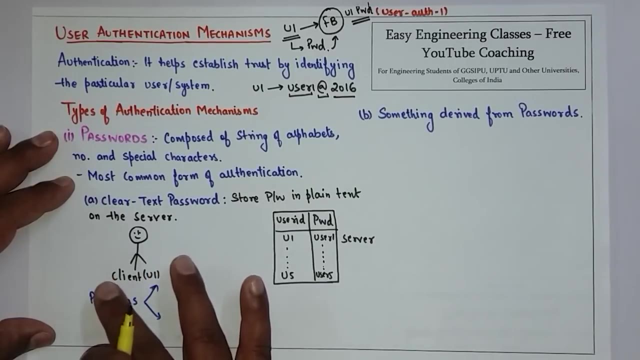 and this client is user1. This is user1. Now user1 wants to gain access to the server, So the user1 has to authenticate himself that he is the right person to access the system by the user1 profile. So what will happen after that is that when user1 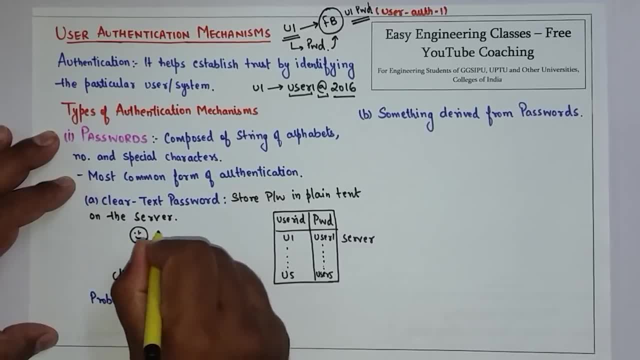 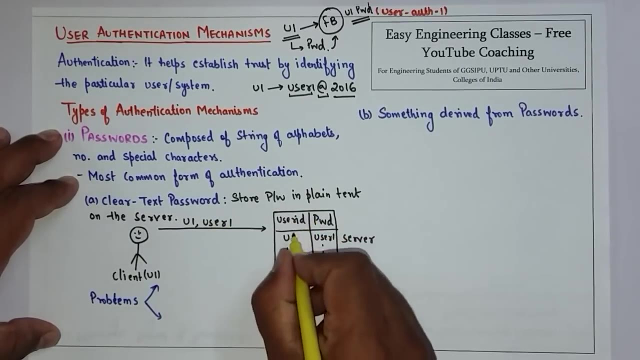 tries to access this server, then a login form opens And in the login form the user enters his details here, Suppose user1, that is, a user ID, and the associated password, which is user1. Now, here what the server will do is that user1 will match the corresponding password of the user ID. 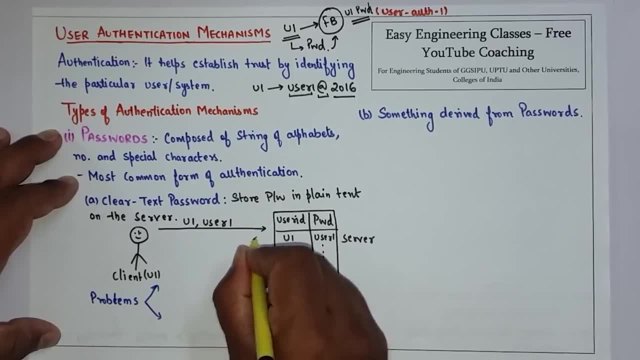 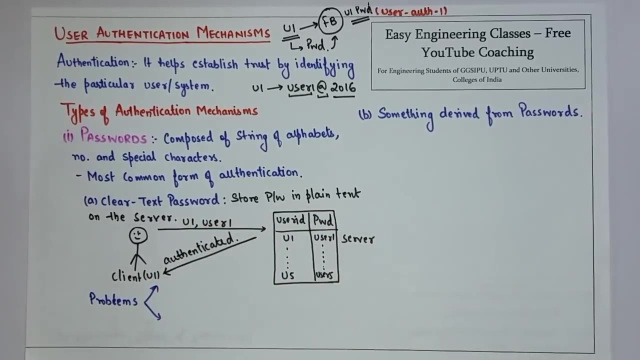 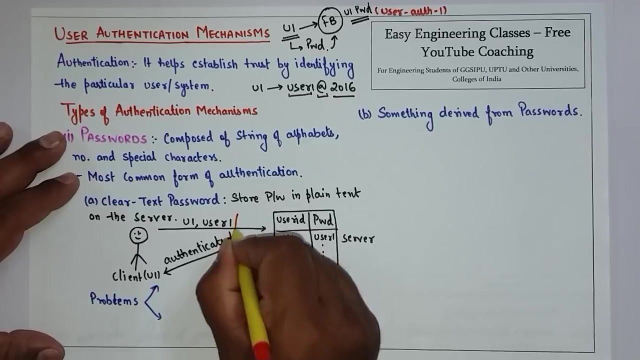 If this and this are same, off by the response will be given back to the client that you are authenticated. if user1 and user1 match, then the message of authenticated will be floated. if, instead of user1, user1 has typed something else like user2, then what will happen is that these two will not match. 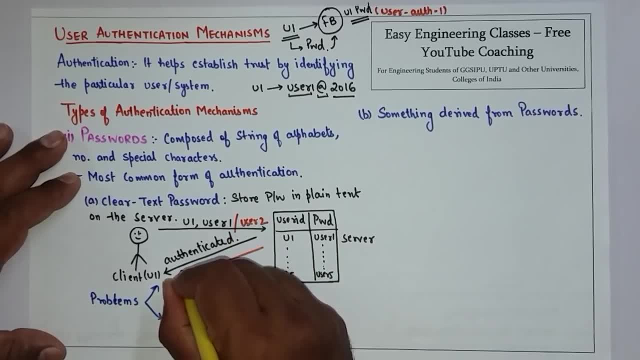 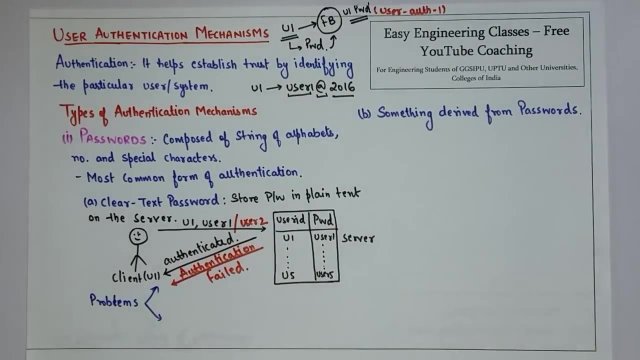 so now what message will come here? authentication failed. so this is a very simple mechanism in clear text password in which server user id's corresponding their password is stored in a simple, plain text form. now see what is the problem. first of all, sorry. first of all, the problem is that 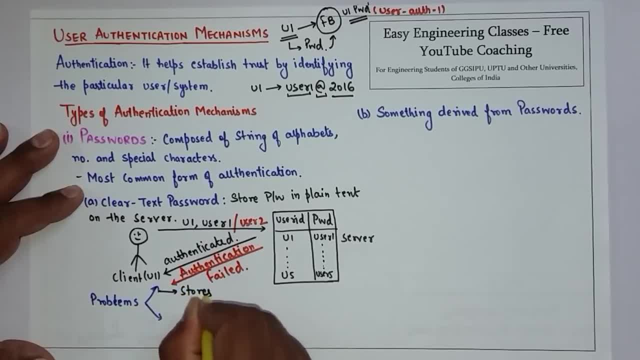 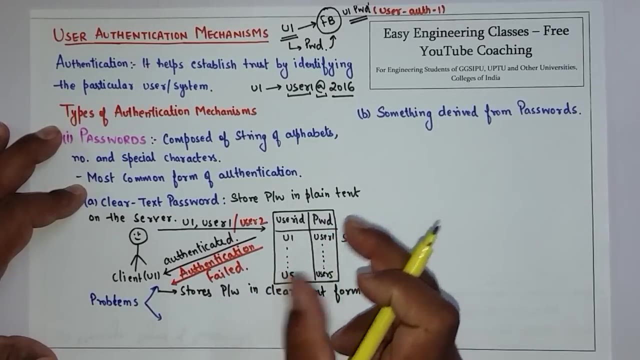 the database on the server that stores the password in clear text form. now, what is the problem of saving it like this? that if ever there is an attack on the server, then the corresponding password of the user id, the details of all of them, is simply stolen by a hacker? 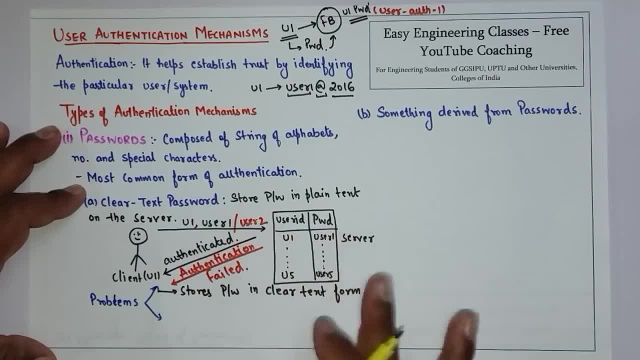 and they can use it further. so this is a problem, that if we keep someone's confidential information in the form of clear text password. second problem is password travels in clear text form from client to server. now what does this mean? as you can see here, the user1. 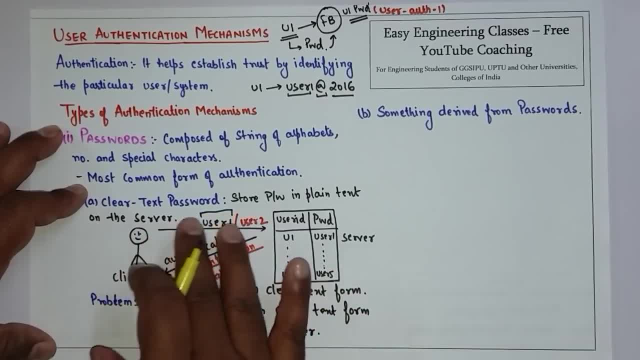 which I am sending the password. it is traveling in the form of a plain text from client to server. now, in between this, there is a route, there are routers and different networks on it. attackers keep their eye, they keep monitoring them and in between this, if any attacker attacks, 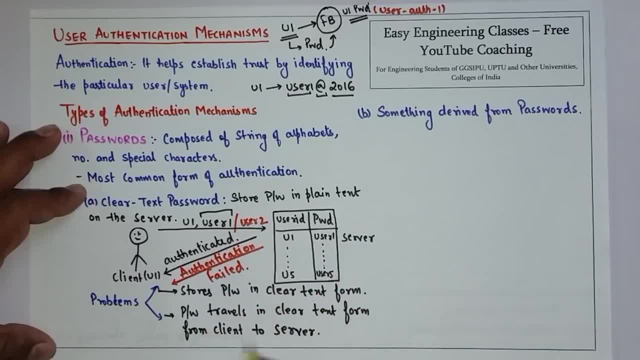 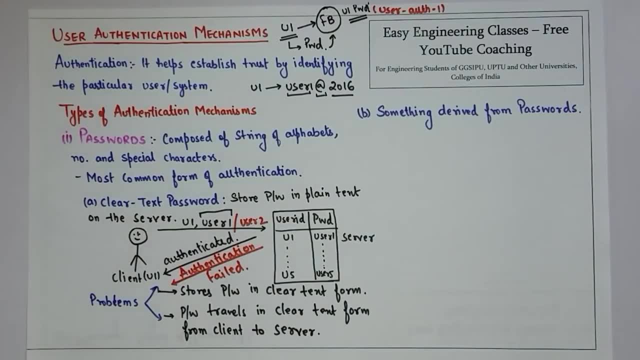 it can easily steal the information. so that is the problem with clear text passwords. so the researchers of different security what did they think? that if we do not store passwords in simple form, but rather they store something derived from them on the server, then it will be more beneficial. 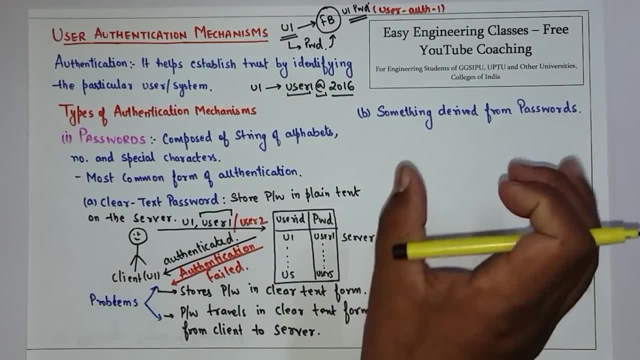 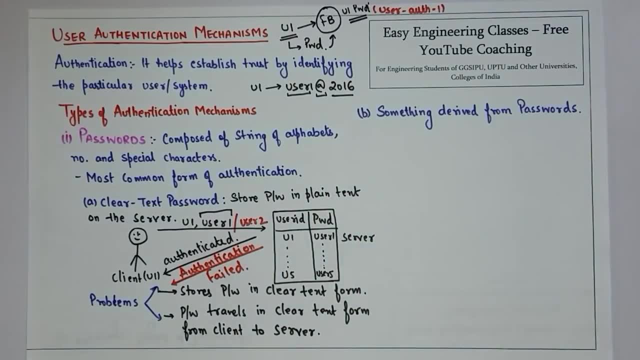 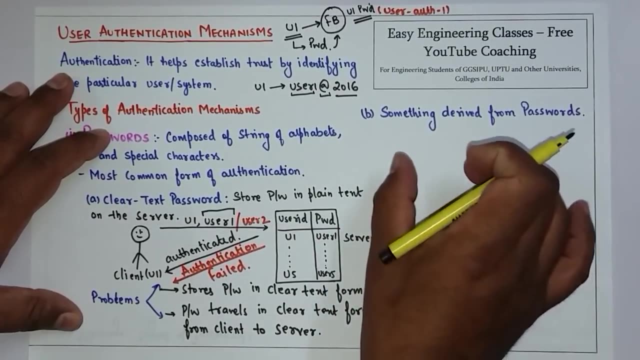 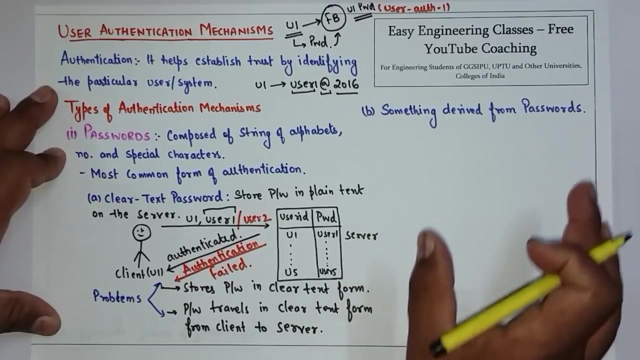 and more secure than clear text passwords. so the second innovation or the second step of password mechanism is something derived from them, something derived from passwords in something derived from passwords. what happens is server runs some kind of encryption process on the passwords and store the encrypted passwords in the database. 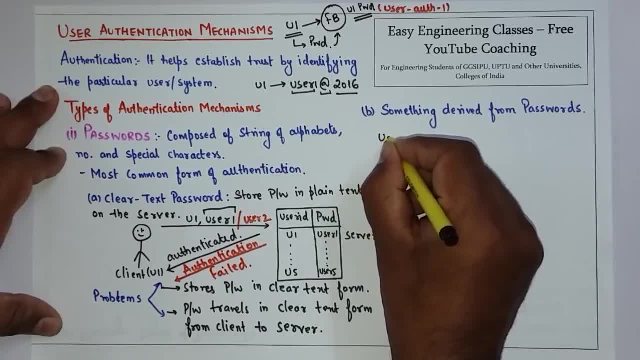 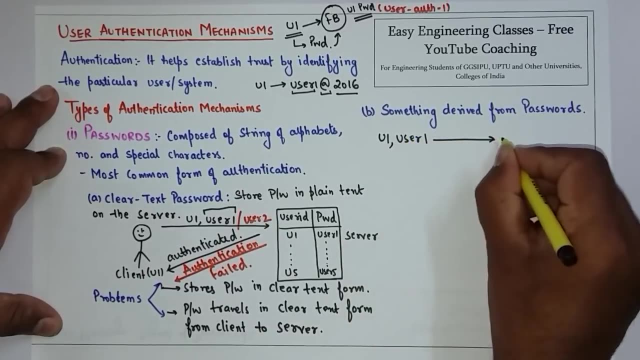 so what happens? is suppose user1 now wants to create a profile on the server. so user1, what will? what he will do is he will send the details in clear text form for the first time to the server. so the details which he has sent were user1 and. 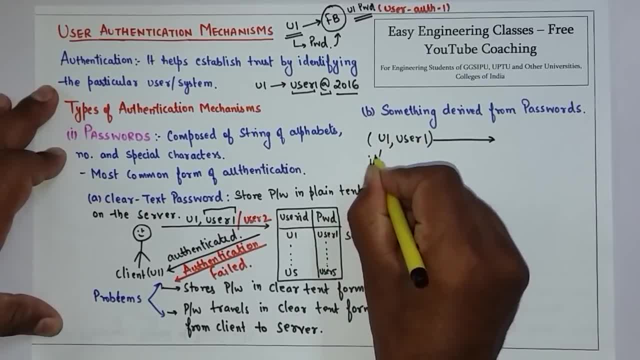 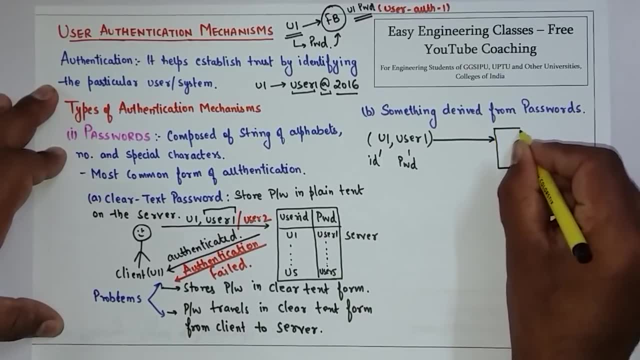 u1 and user1. this is the id and this is the password. now what will happen on the server? server will first pass it through an encrypted program. now that encrypted program will translate this user1, which is the password, into an encrypted form. suppose the translation is now. 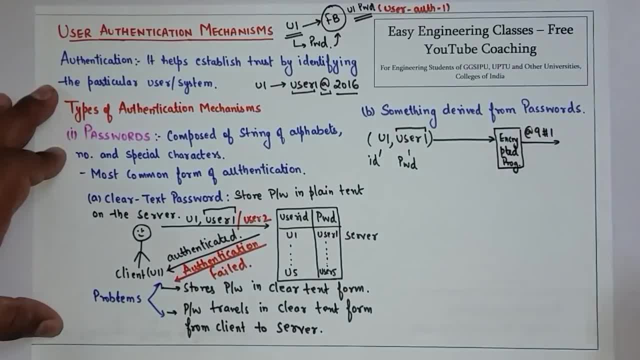 at the rate 9 hash 1. we have now converted user1 into this form. now in the database the password which will be stored for user1 will be at the rate 9 hash 1, at the rate 9 hash 1, 2, and so on. 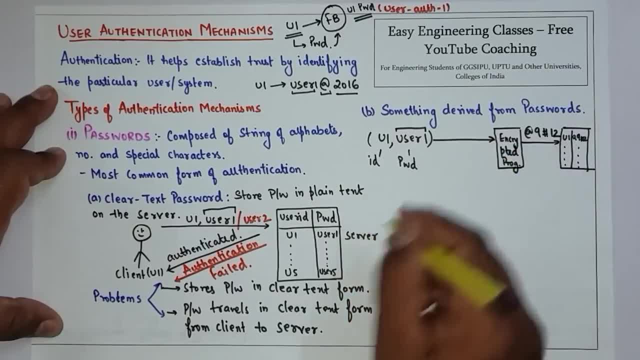 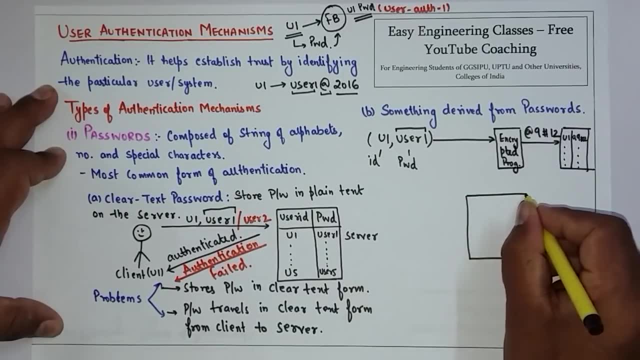 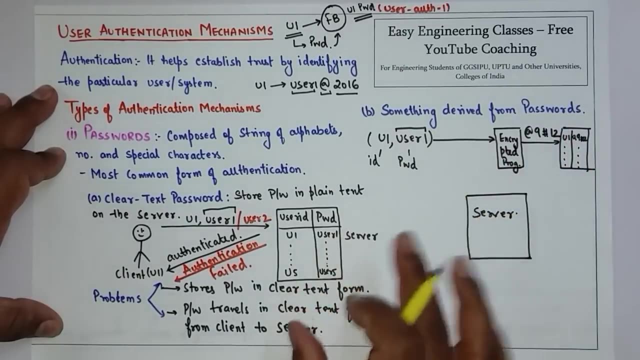 so this is the first time that the user has created the profile. now, what will happen after that, when user1 has to login again in the system using this particular mechanism? this is the server now. there are two scenarios in this. one scenario is that user1 has sent his details. 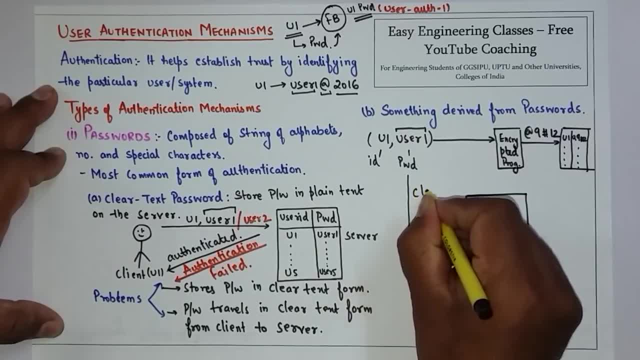 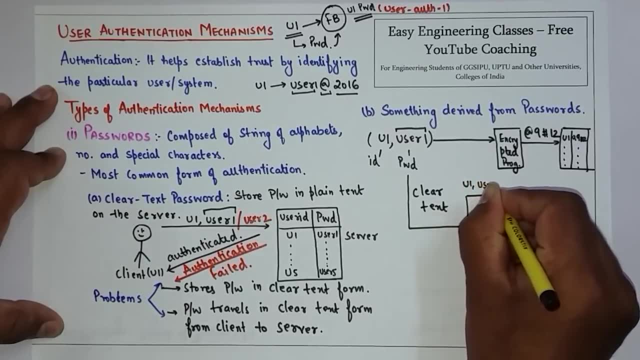 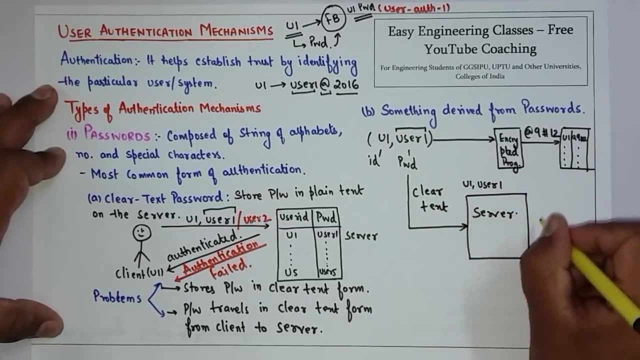 in clear text form. in clear text form to the server. now, what did the server get here? u1 and user1. now server wants to authenticate whether this is the correct information or not and what is being stored in the database of the server. u1 at the rate 9 hash 1, 2. 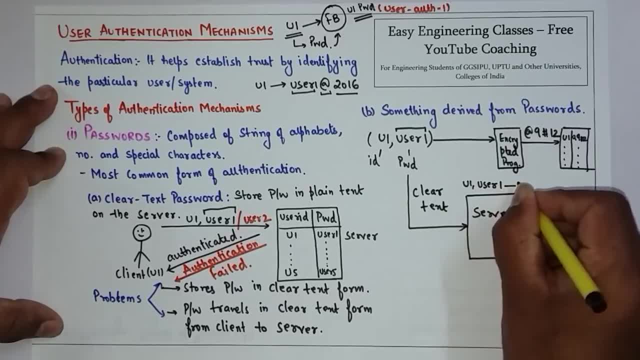 so what will server do is server will again pass this password to the encrypted program and then check whether the encrypted text is valid or not. now the encryption of user1 will be same at the rate 9 hash, 1, 2. so the message that will: 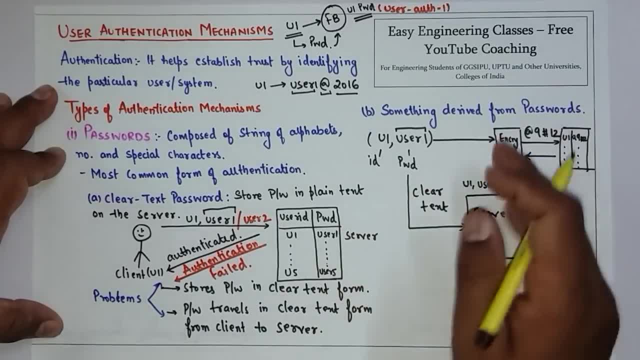 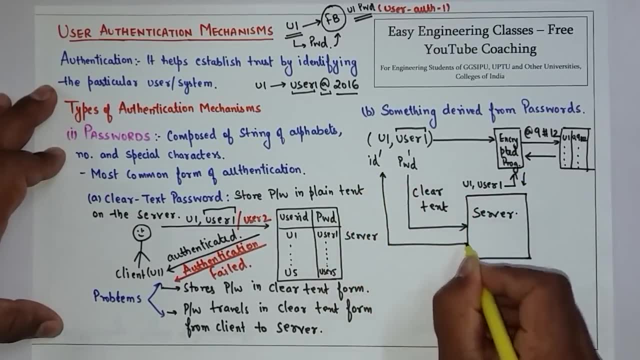 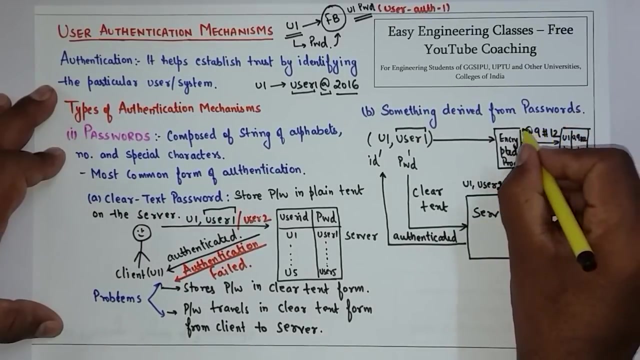 be passed from the database to the server and finally to client, is that you are authenticated to access the program. so this is the correct authentication. now in this, if we see instead of user1- if he had written user2 here- then the encrypted text which is converted here: 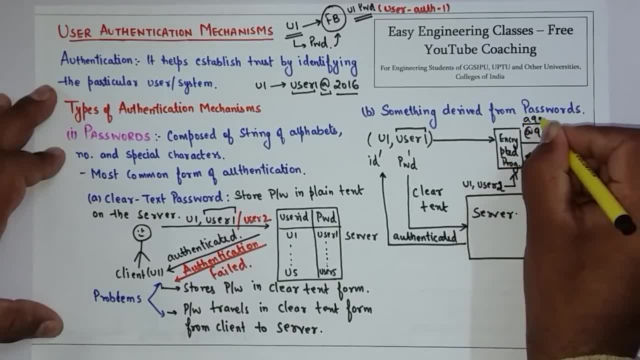 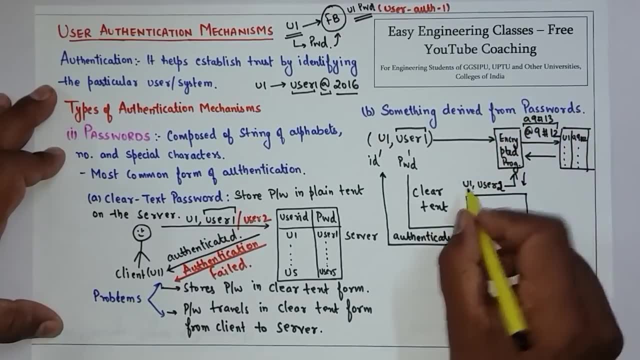 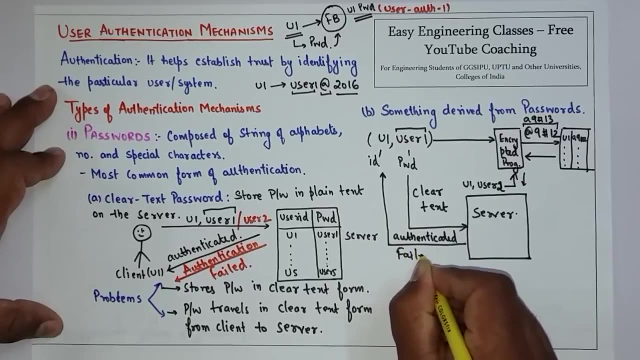 will be something else. for example, at the rate 9 hash 1, 3. now if you match this with this, then it will be incorrect. so if user1 had given user2 password, then in that case it would have been authentication failed. so one scenario is that 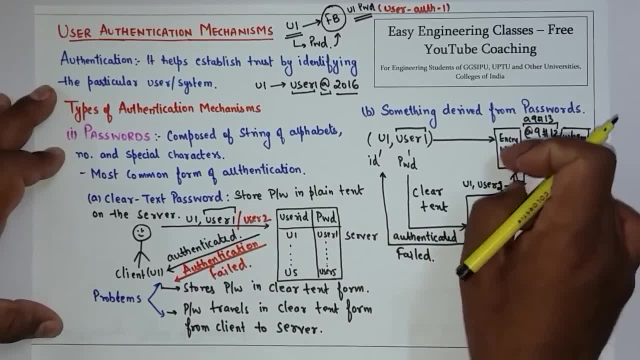 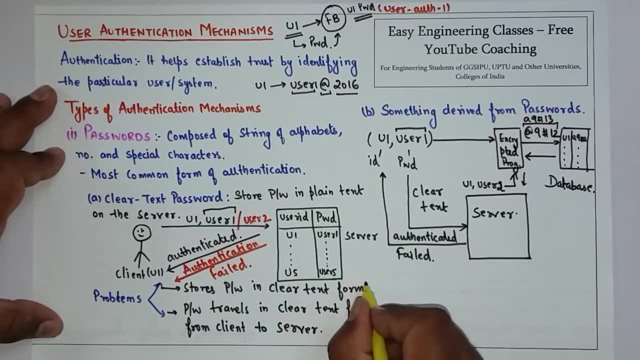 user is sending the server in the form of clear text, server is encrypting the password again from the database. so with this mechanism our problem is solved, in which server made a mistake in keeping the password in clear text form. in this mechanism, here we are keeping the password. 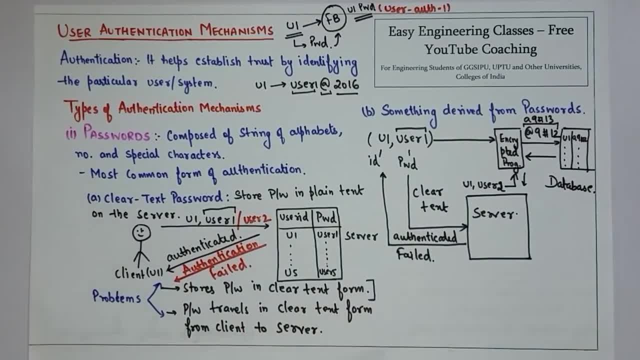 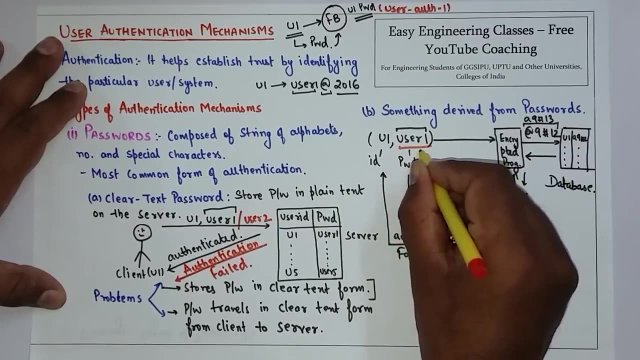 in encrypted form, but this problem, that password travels in clear text form, is still there. so for that, what can be a variant in this system that whenever the user wants to authenticate user runs the same encryption on the password string on their client machine? now, if here itself, 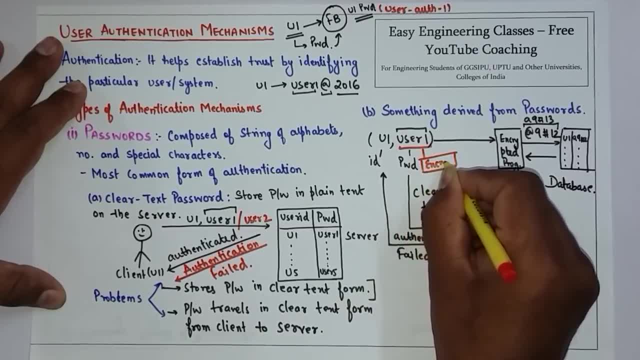 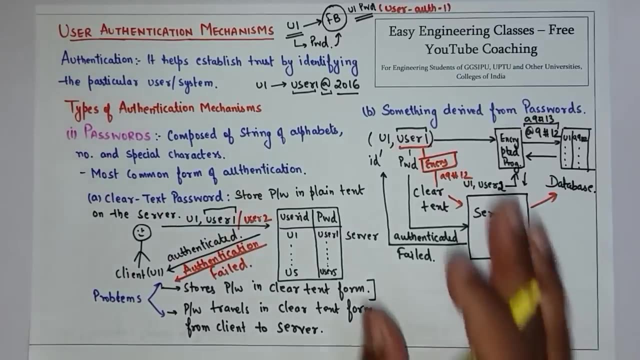 the same algorithm of encryption is implemented here. he has encrypted it here. it was generated at the rate 9 hash 1, 2, and now it has come to the server so the server can directly check it from the database. so if you in something, drive form password. 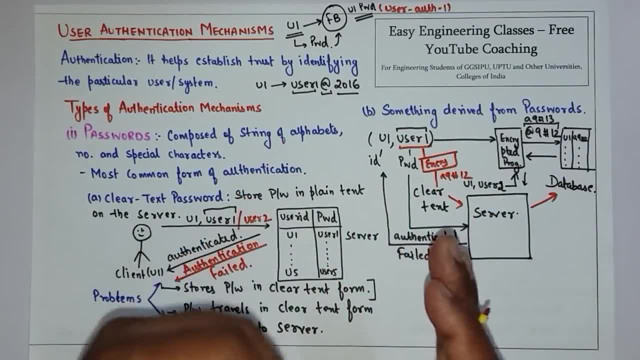 if you install the encryption module on the client side somehow, then the problem of password travels in clear text from client to server will also be resolved. so this is about how you can do the authentication mechanism using something derived from passwords. the next variant of using password sets: 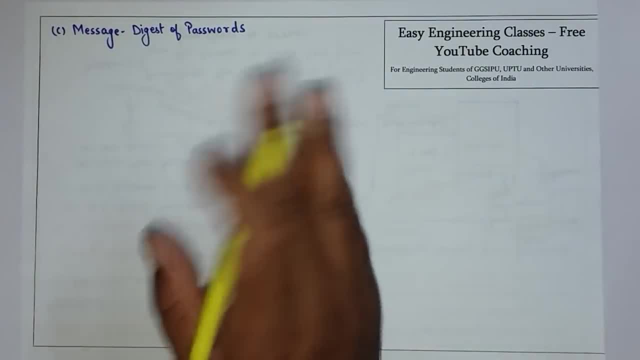 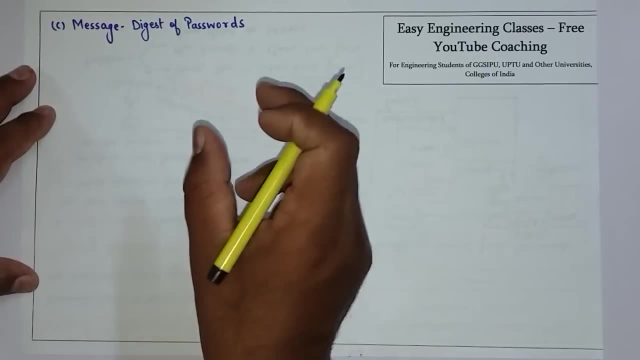 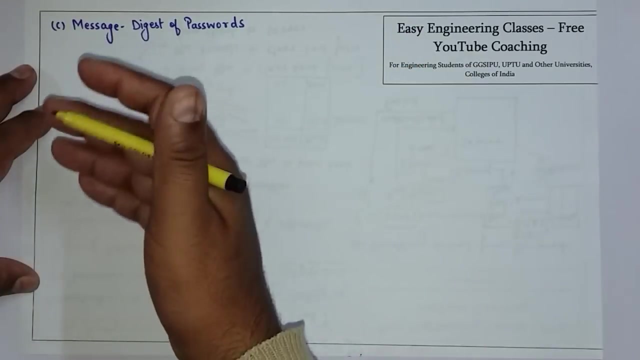 the authentication mechanism is actually using the message digest of the passwords, like we have seen in simple derived something from password case that we were installing some encryption algorithm and that encrypted password we were storing in the database. instead of that, what we can do, we can also use message digest. 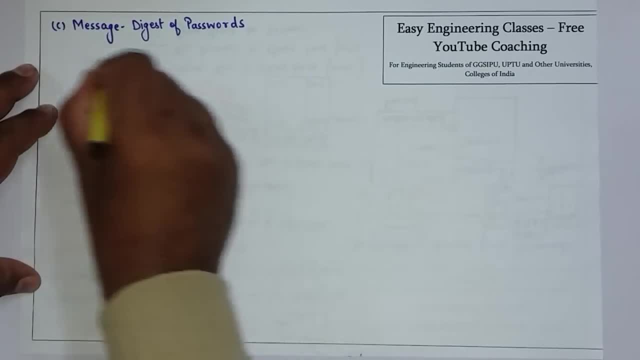 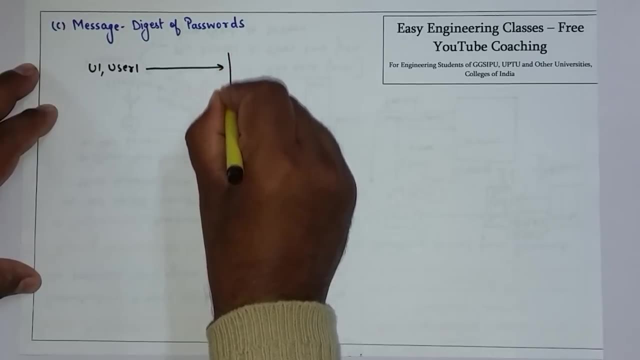 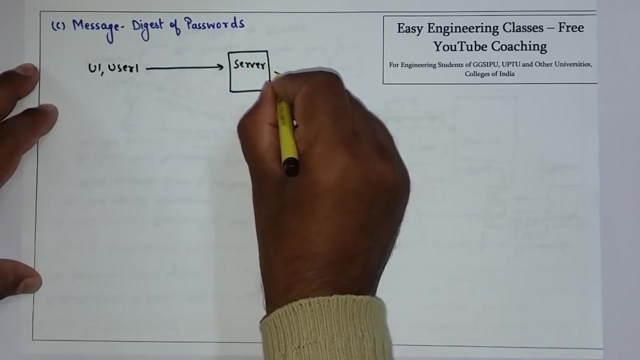 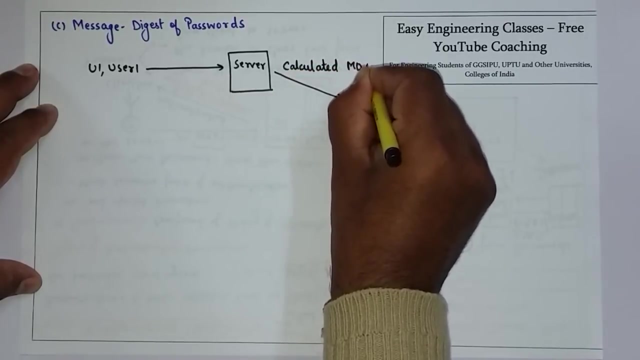 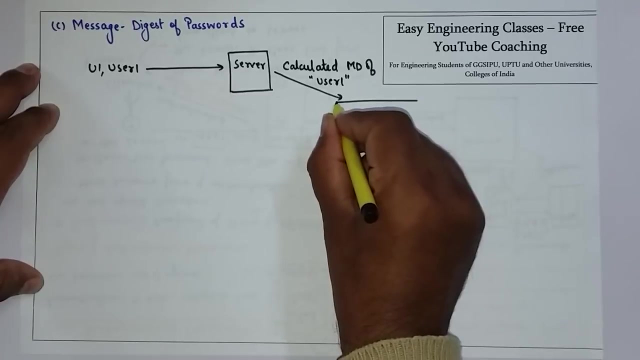 so now in this case what happens? that the user suppose user1 and user1, this information goes to the server for the first time. server calculates the message digest of it, calculates message digest of password string which is user1 and store that message digest in the database. 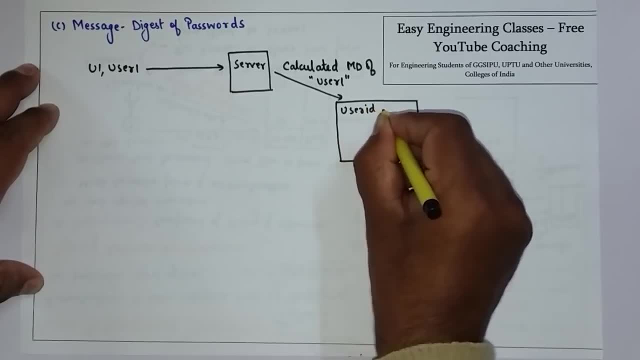 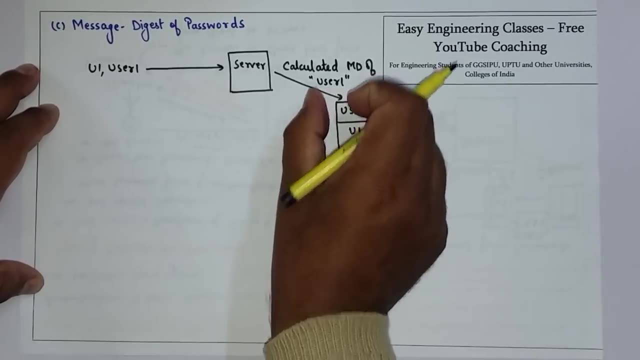 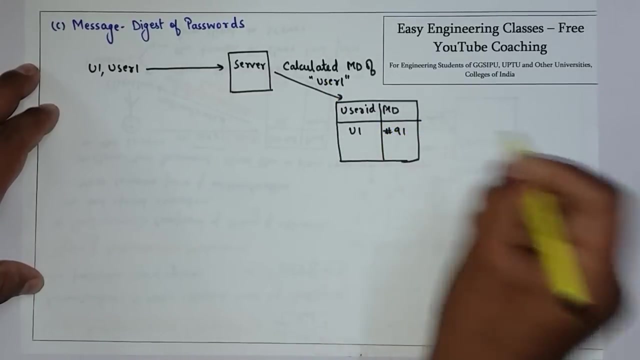 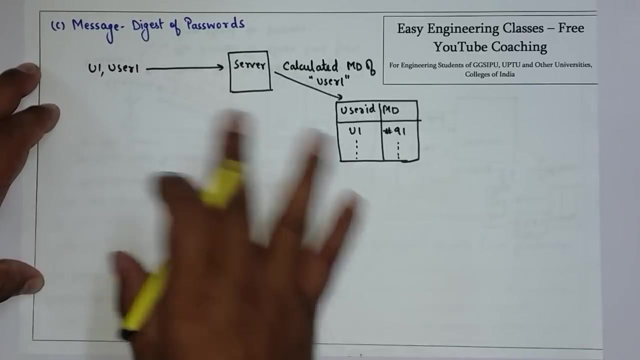 so what will happen here? there will be a table, suppose userid, and md, suppose message digest. so the corresponding of user1 and its message digest will be stored, for example, hash91 and so on, for other users. this is the first time the user has created his profile. 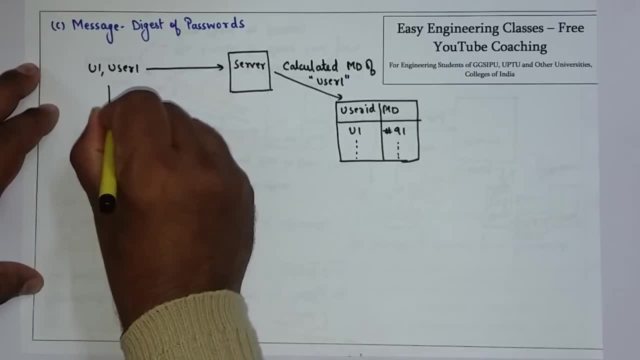 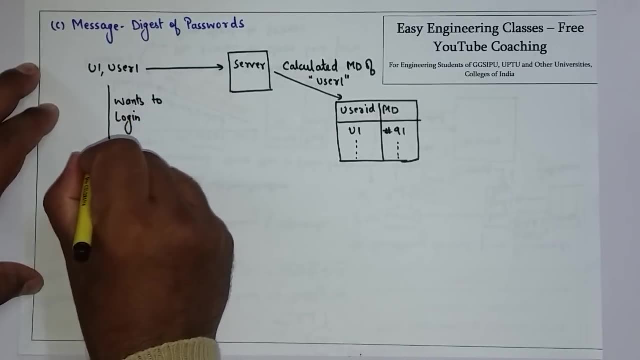 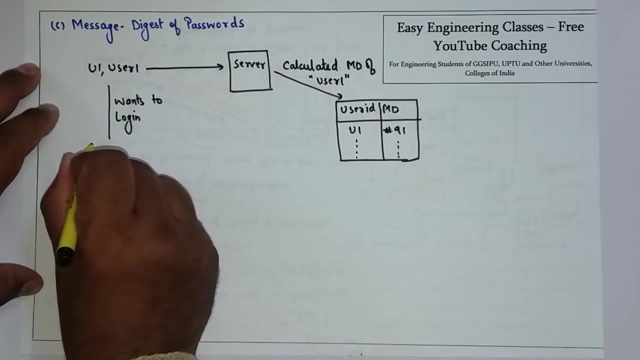 now the user has to login. so the user wants to login, wants to login. so what will the user do? user will calculate the message digest on the client side. so what the user did? he calculated the message digest of user1 here. this is the message digest and after calculating, 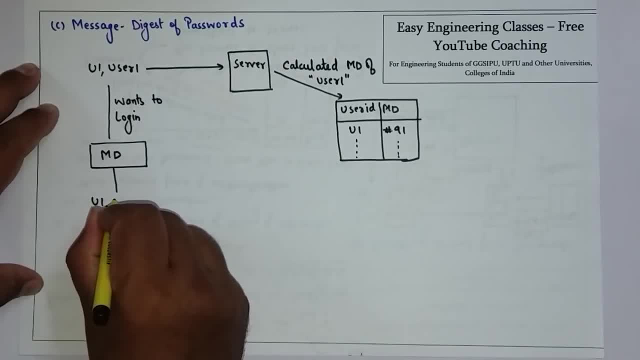 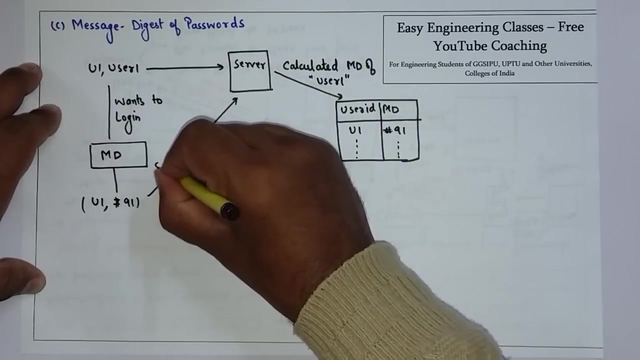 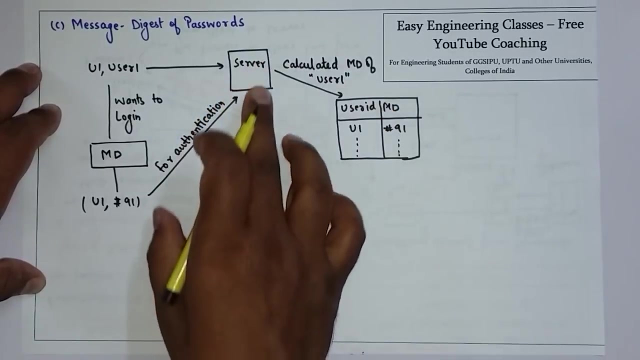 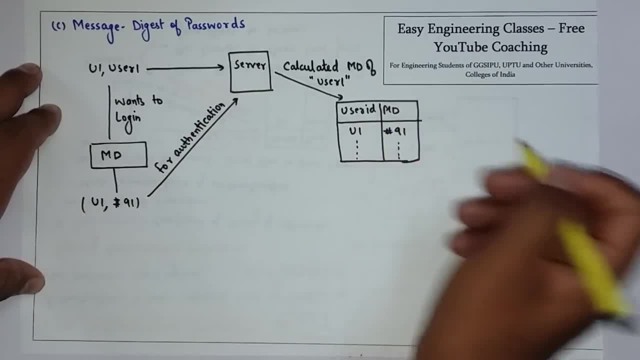 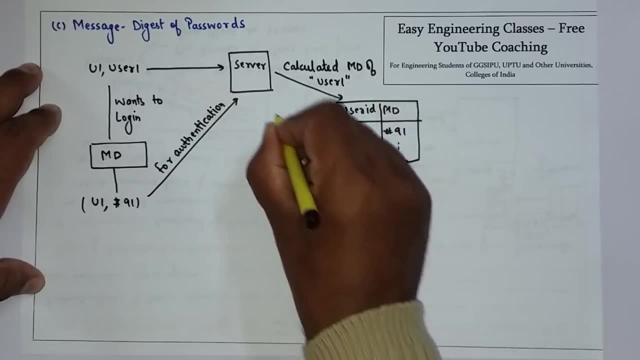 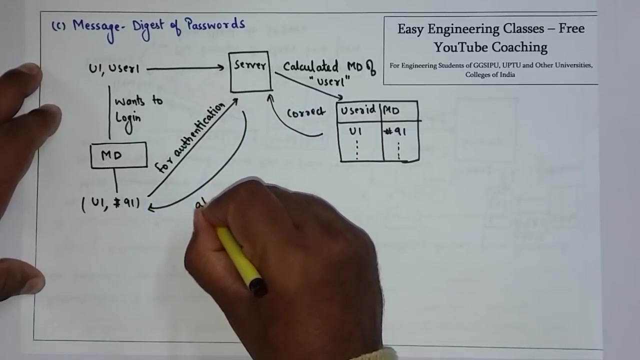 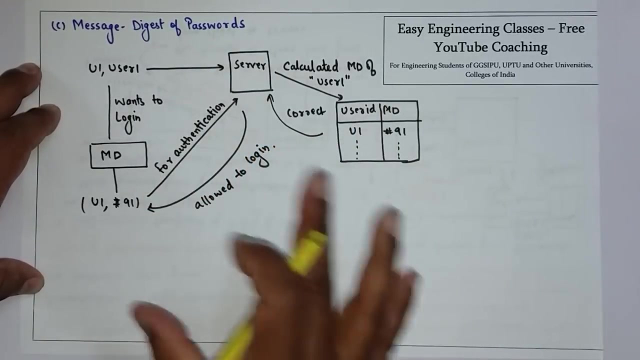 has the associated message digest as hash91. if the same string is find out in the database, then the response will be send at correct and from server to user allowed to access or allowed to login. so this is the very simple process of using message digest as encrypted form of passwords.